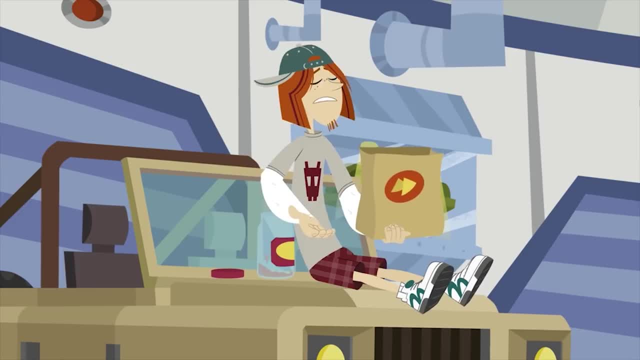 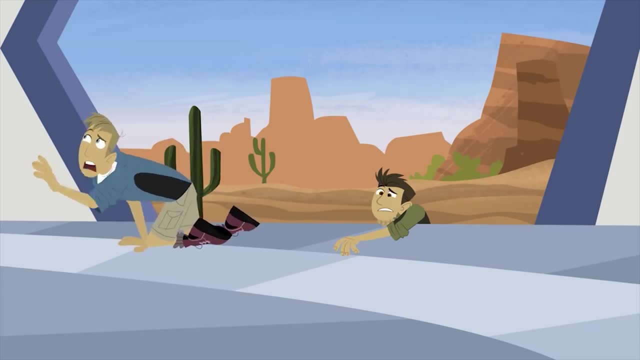 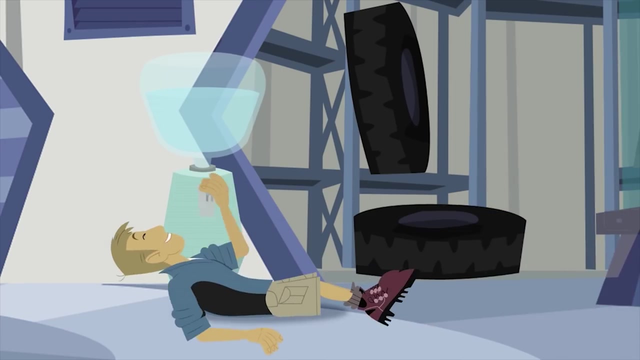 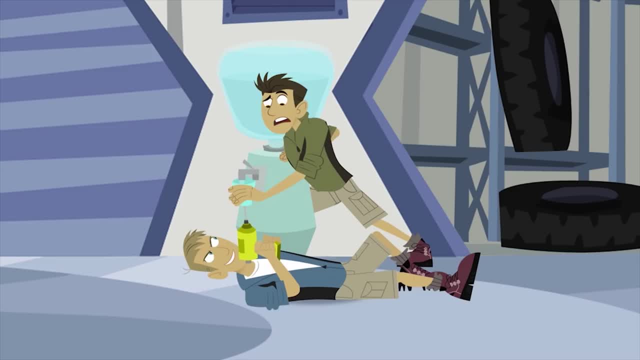 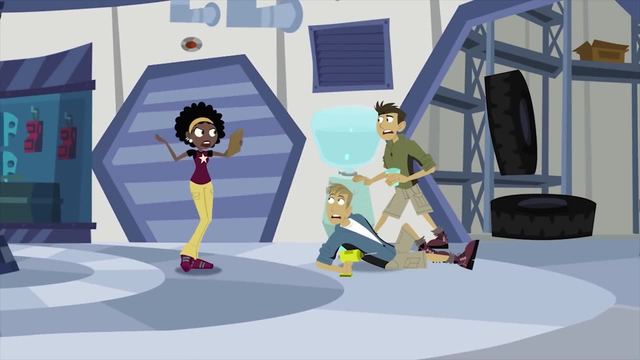 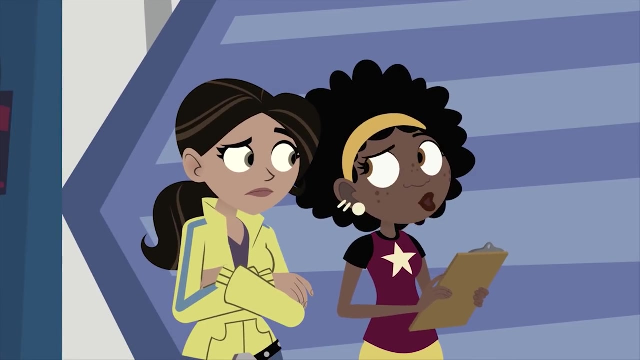 Hey gotcha, Huh, Guys, knock it off. We have to conserve. This is our last bottle of water. Aviva and I have just decided we have to leave now and go to town and get resupplied. What? 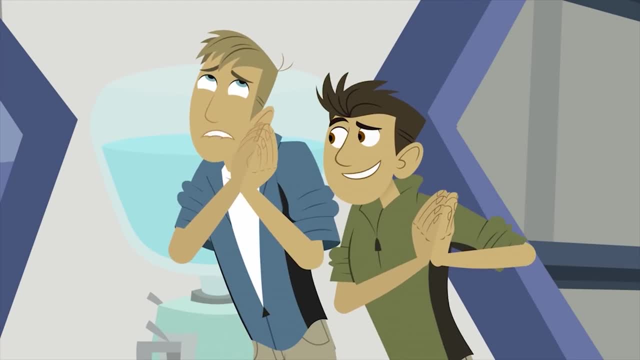 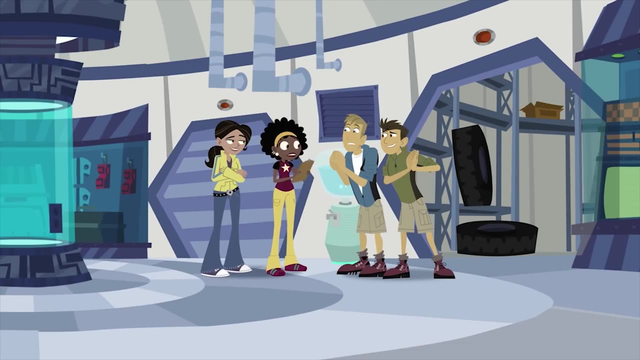 But we just got here to the Sonoran Desert and we've only met a few of the creatures who live here. I told you I know, but we've run out of so many things and Oh no, This is the last bag of nachos and we have no more salsa. 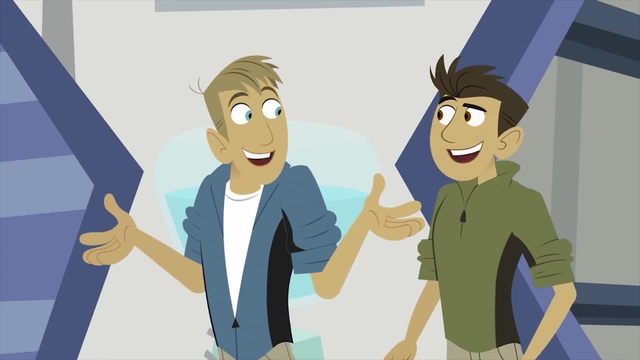 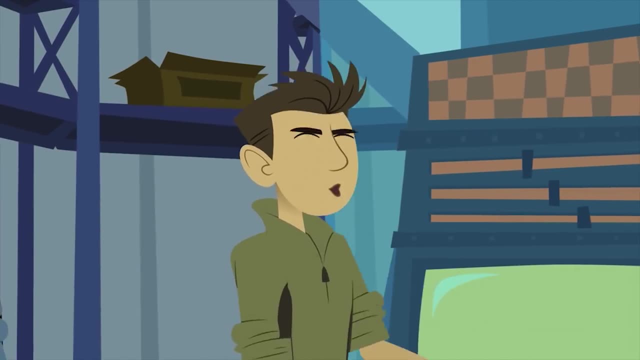 Oh yeah, you do have to have salsa for your nachos, especially when you're adventuring in the desert southwest. Wait a second, We can't go now. We're just on the tail of that speedy little mystery lizard over there. 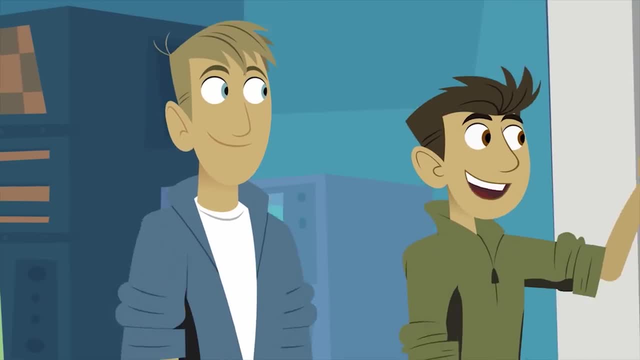 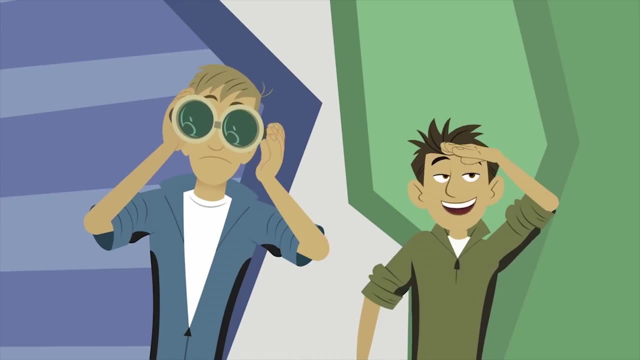 Leaving now is against the Wild Kratts, Creature Adventure and Code of Conduct. Yeah, you're right, bro, We've got to stay until we know exactly who that mystery lizard is. Whoever it is, it'll be a new animal for our life list. 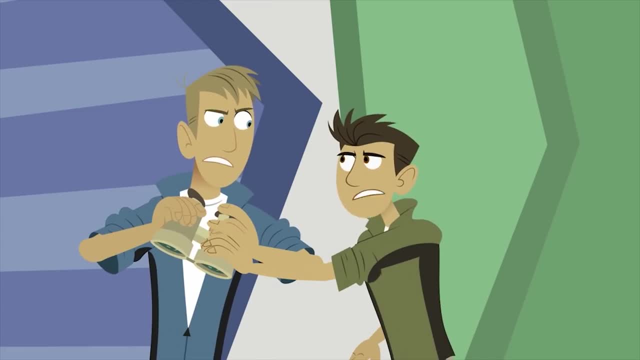 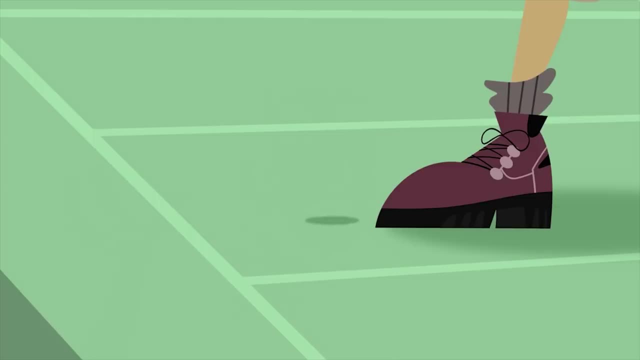 Sing through binoculars Doesn't count. We have to see it up close and personal. to add it to our life list, I know, but at least we know what we're trying to get a closer look at. Oops, Whoa. 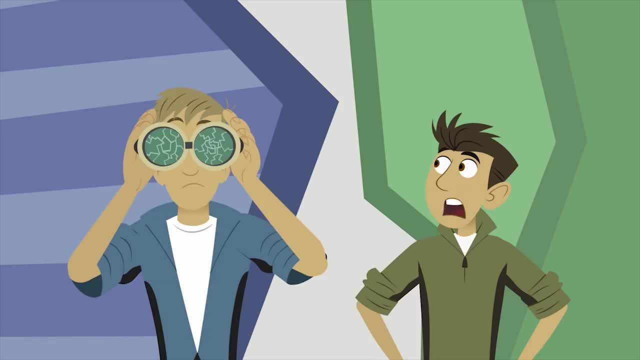 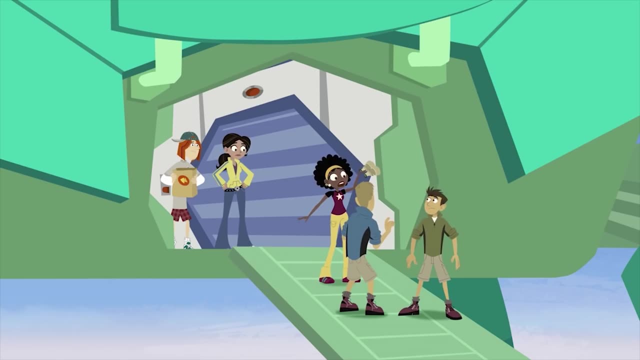 It has two tails, three eyes and, uh Martin, The binoculars are broken. Now we have another reason to head to the nearest town: New binoculars. Come on, guys, get packed up and ready to go. 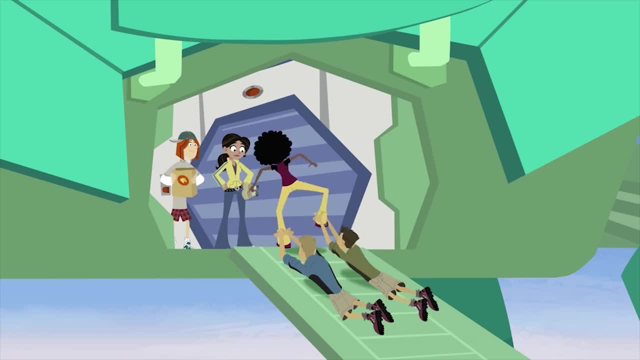 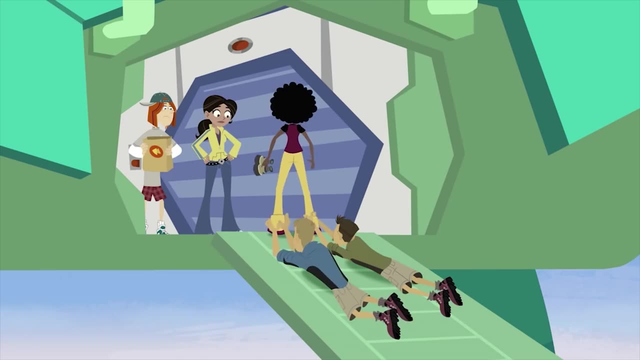 Please, Just five more. Five more minutes. Oh, come on, We just have to get close to that speedy mystery lizard. Just five more minutes, Please, Please. Fine, I still have to realign the Tortuga's hover thrusters before we take off. 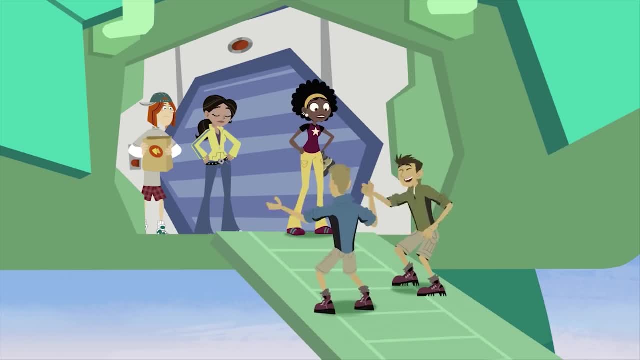 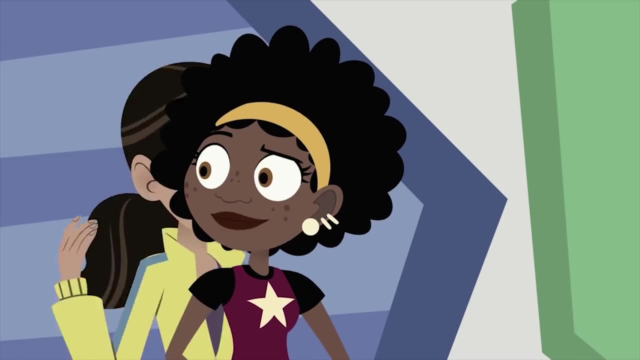 I can give you half an hour. All right, Yeah, All right. Hey, Thanks, Koki. Yeah, we'll be right back. Sure, you will. All right, This'll be great. As soon as I spot the lizard, I'm ready to go. 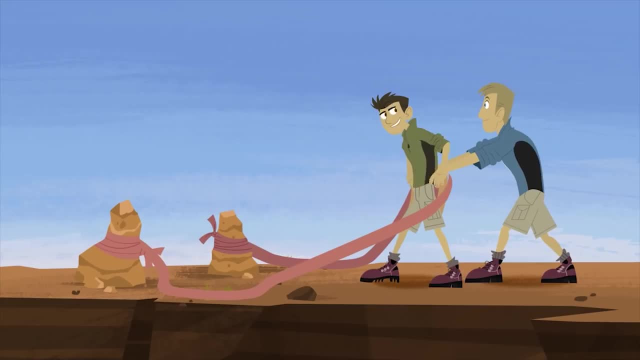 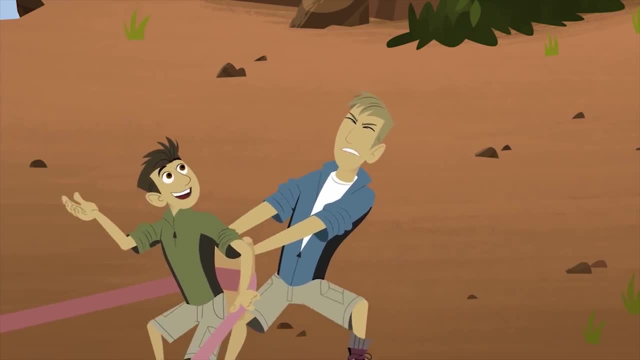 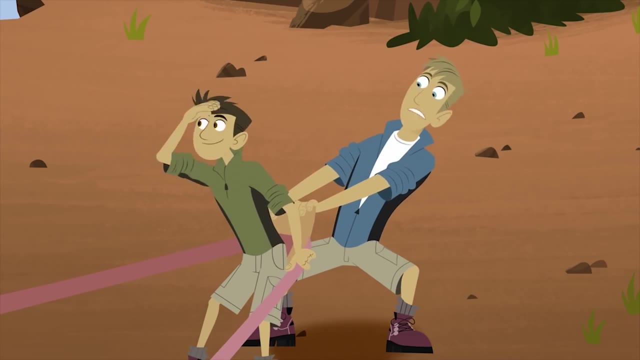 You see the lizard, Not yet Could be a while. Oh, there he is, Whoa, Whoa. You scared me, Lizard, What? No, I'm scared, I'm scared. You scared me, I'm scared. 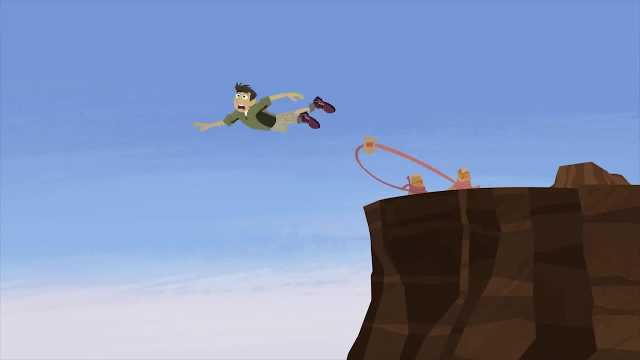 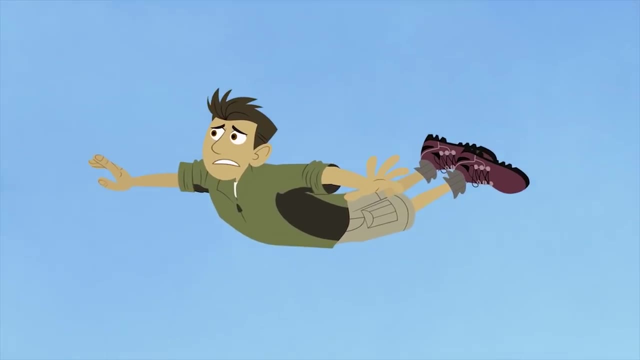 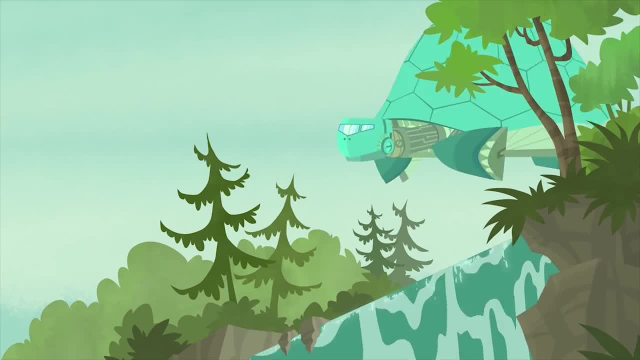 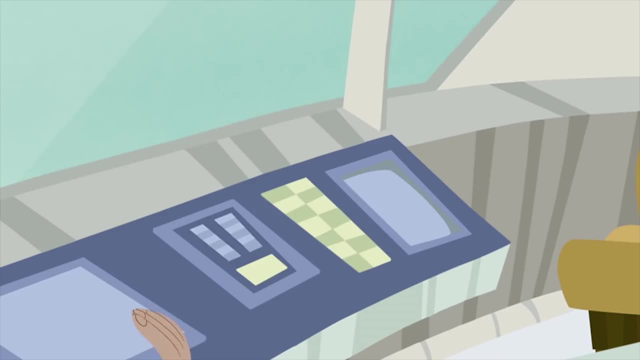 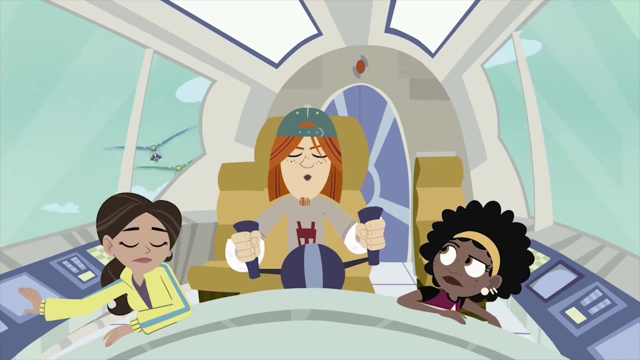 Give it all. you got, You got it. Whoa-ho. This is not the way to see North America. You can say that again. Smooth it out, Jay-Z Slower. A few more turns, I'll give him the old Jay-Z jigsack. 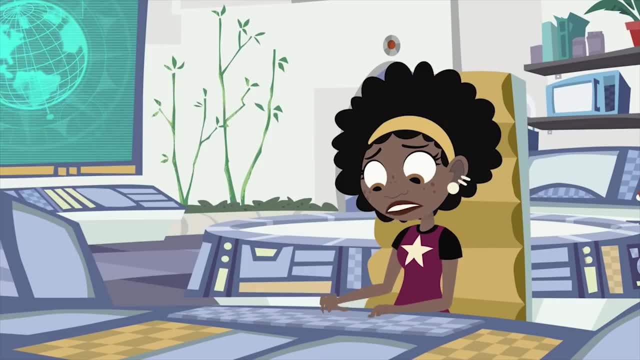 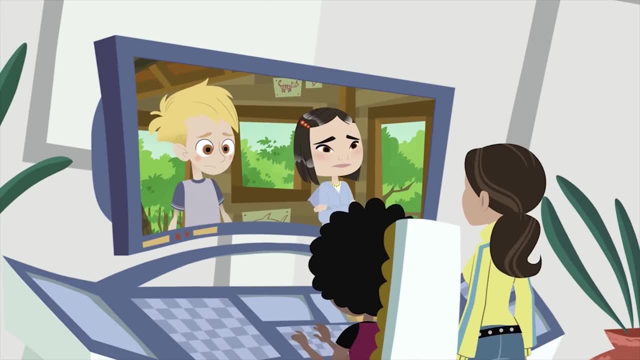 A creature alert Coming in from some Wild Kratts' kids Um in eastern North America, Wild Kratts' Tortuga HQ Mystery, discovery or rescue Mystery, I guess. Wait no Rescue, Wait maybe all three. 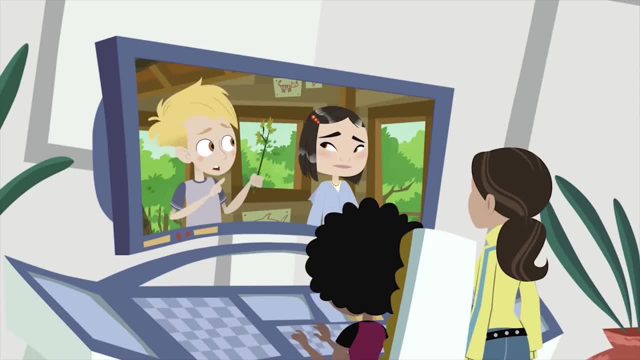 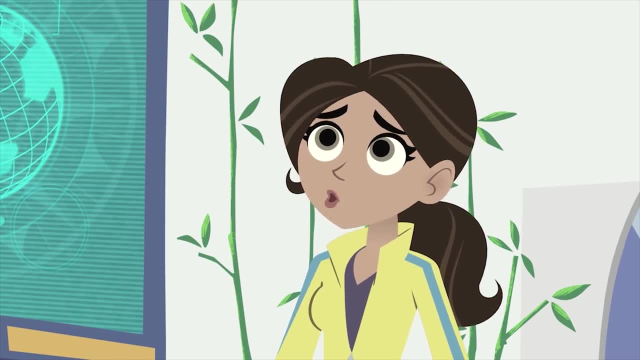 Wow, what's going on? We've got a big problem. Our clubhouse tree is dying. Even worse, The whole forest here is dying. What? All the trees are dying, Why, We don't know. We're worried about all the creatures that live here too. 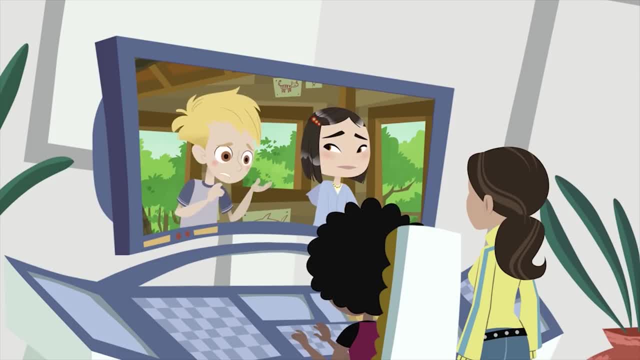 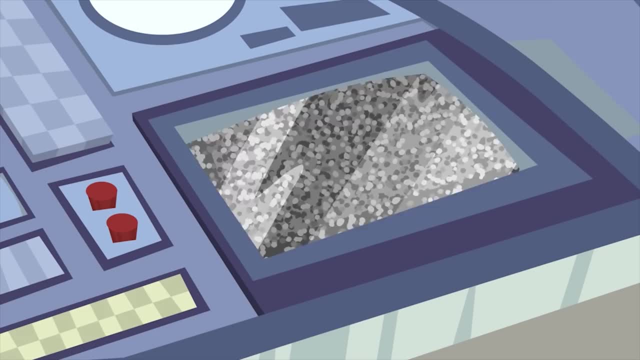 They can't live without their forest. See, It's a mystery And a rescue All rolled into one. We need help. You're not kidding. Hang tight, We're on our way, Jimmy, take her down Double speed. 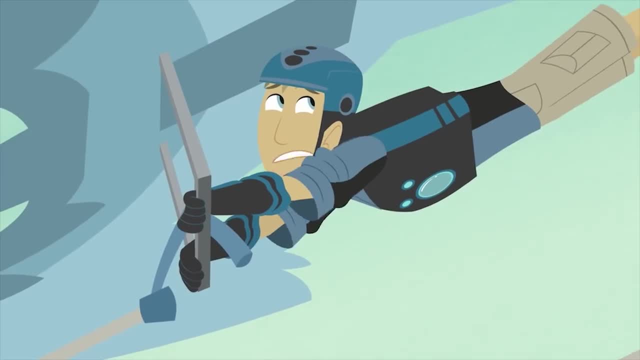 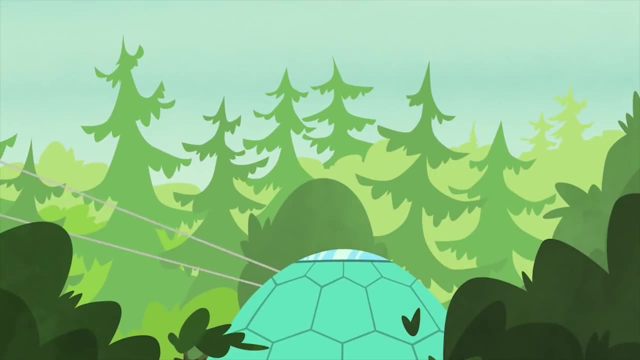 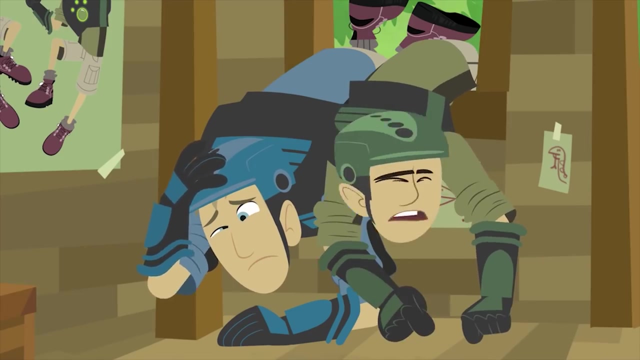 What's going on? Whoa? Did you tell him to give it all he's got? I didn't know he had this much. Yep, That hurt Brr. Oh, hi guys. Um, the door's over there. 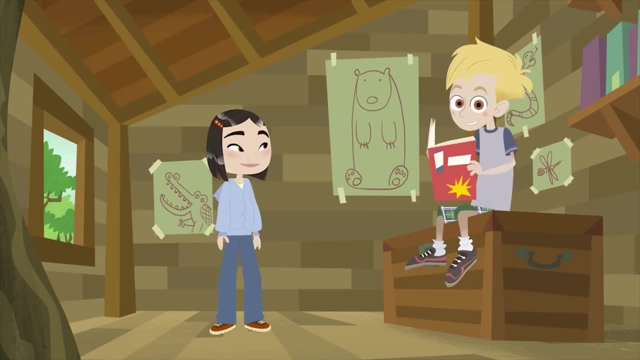 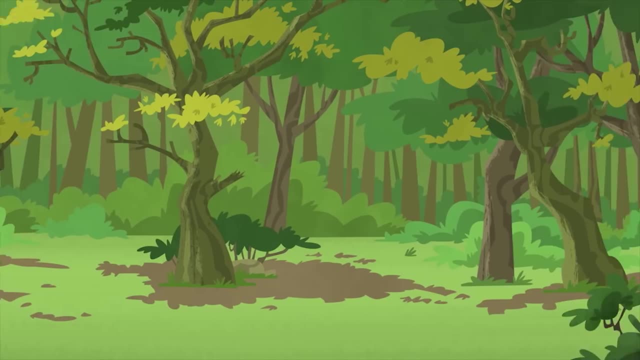 Uh, that's okay, Window will do. Boy, are we happy to see you guys? Oh yeah, What's up? See, It's the trees. They're losing their leaves in the middle of spring. They're sick and we don't know why. 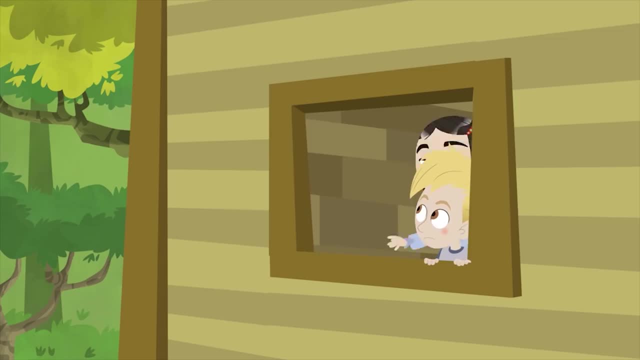 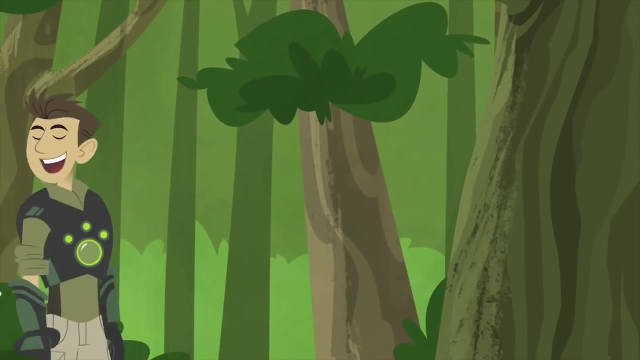 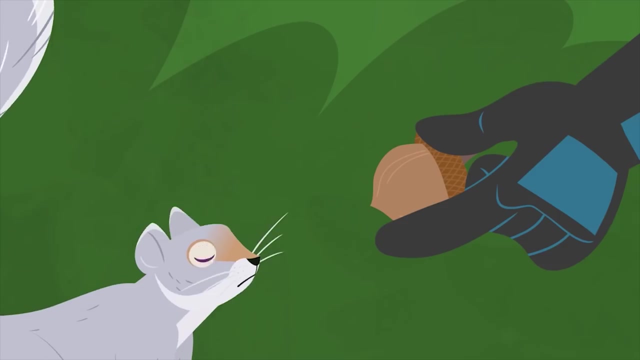 Wow, Not good. Thanks for the alert, Aiden. We're on the case. We'll figure it out. Okay, First we gotta inspect these trees. I'll do a check up top, With a little help from this guy. 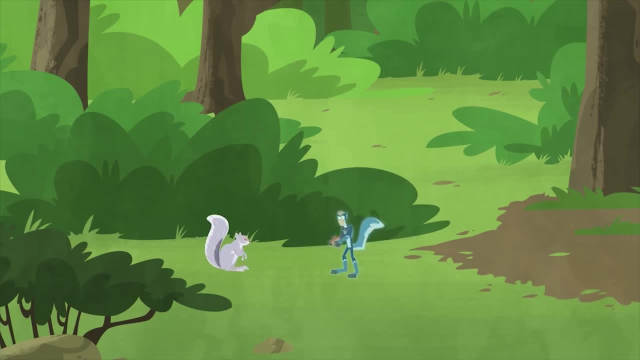 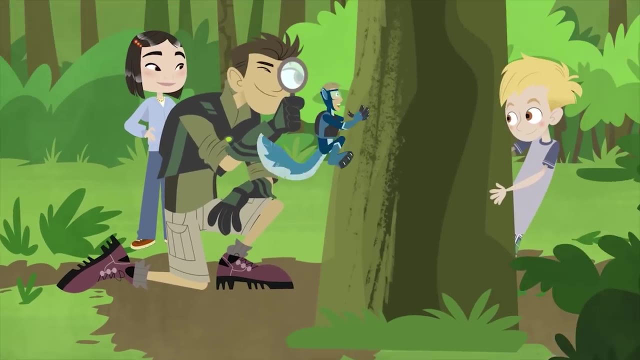 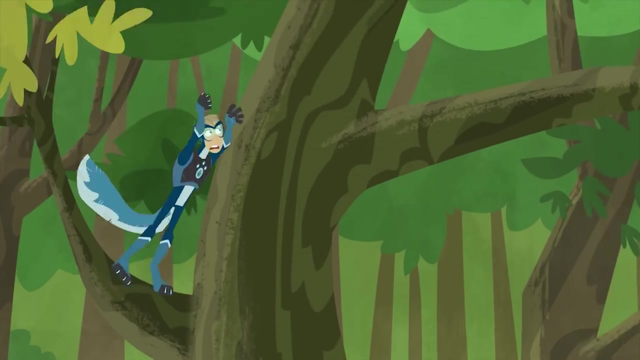 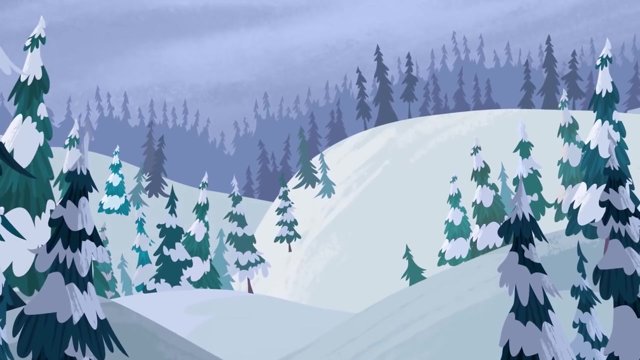 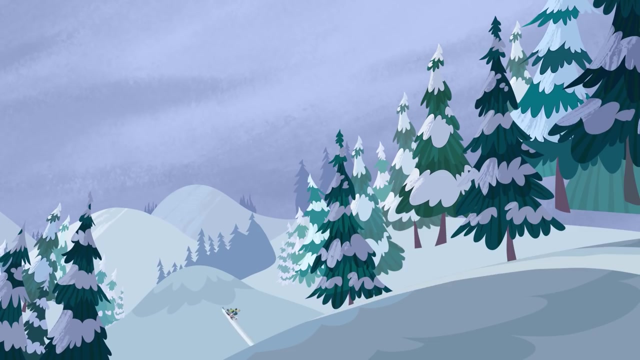 Activate Squirtle Power, Ready to climb? Hmm, Nothing unusual here on the trunk. Hmm, Nothing strange here, Or here, Or here. Yee-haw, Ha-ha Told you these rocket jets would take sledding to a new level. 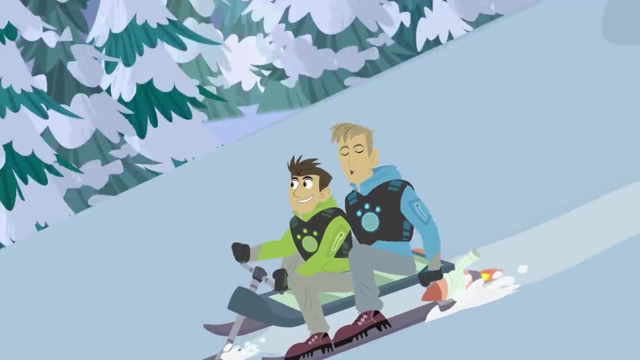 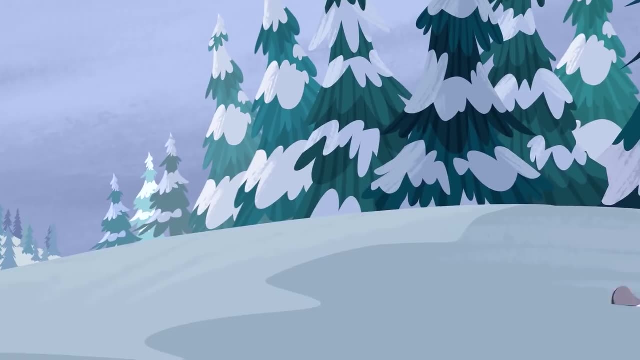 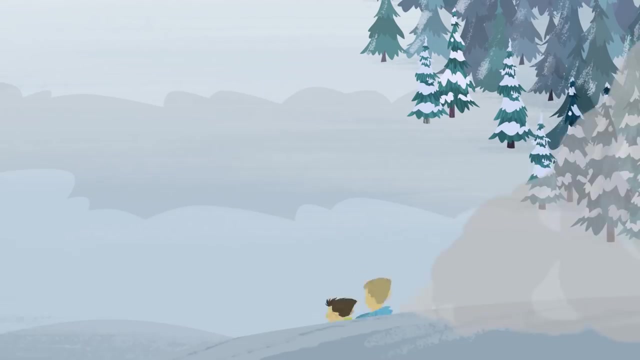 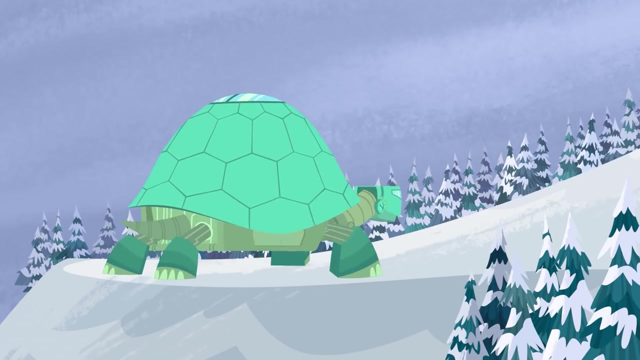 Woo-hoo, Oh yeah. Way to lash on the jets, bro. This is awsome. Woo-hoo, Yeah, Woo-hoo, Woo-hoo, Diff Blast. Righty-o, The Tortuga has lived. They're supposed to be somewhere around here. 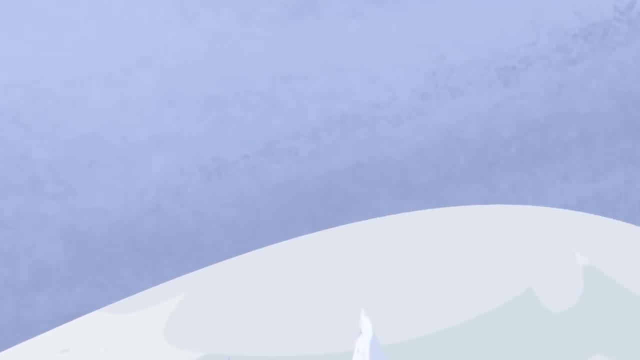 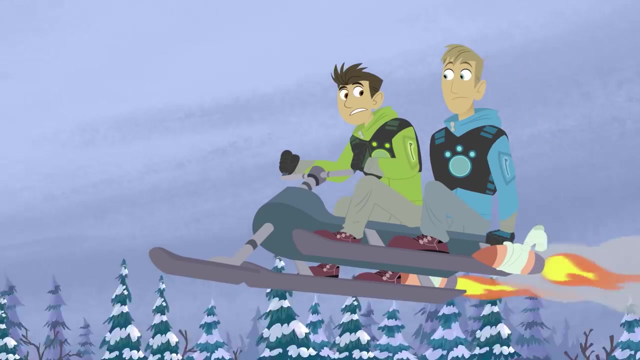 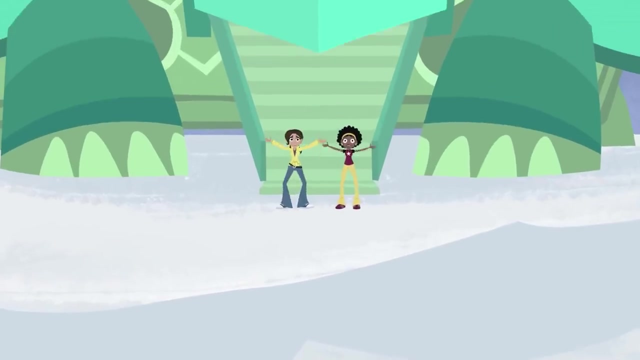 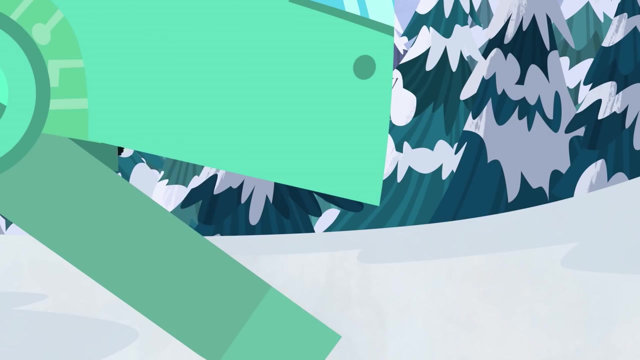 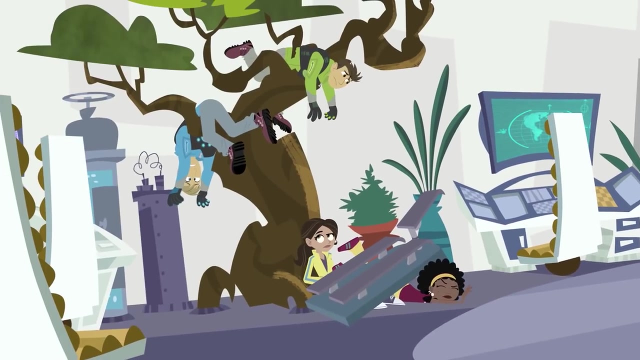 Well, I don't see them Now. do you see them? Whoa, Uh-oh, Got the jets. Whoa, Whoa, Stop. We can't Whoa Run. Oh Uh, How's that for a stop? 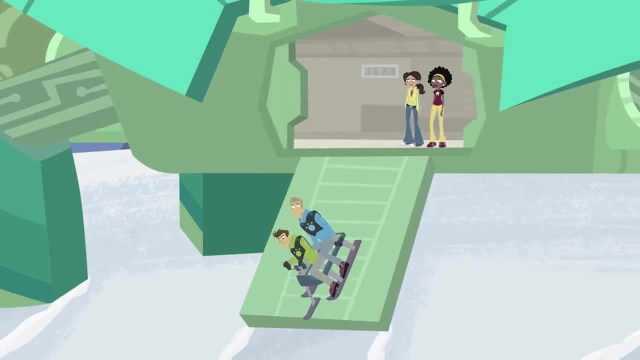 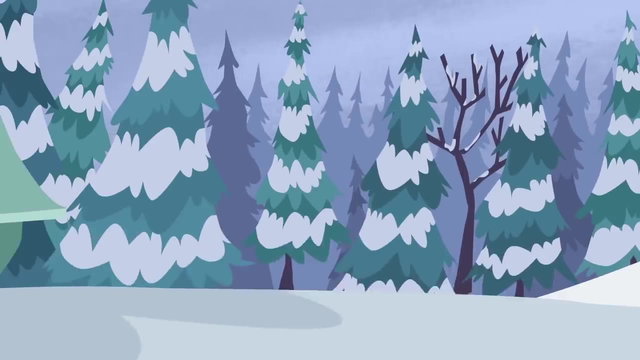 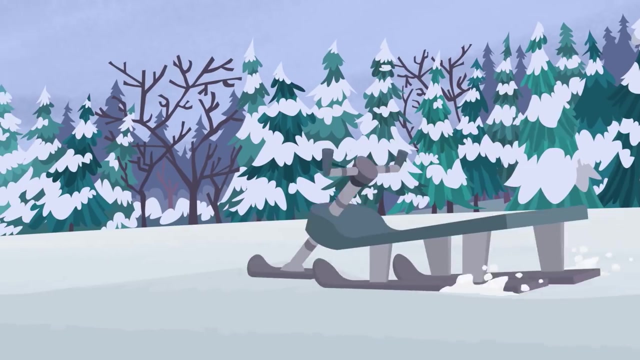 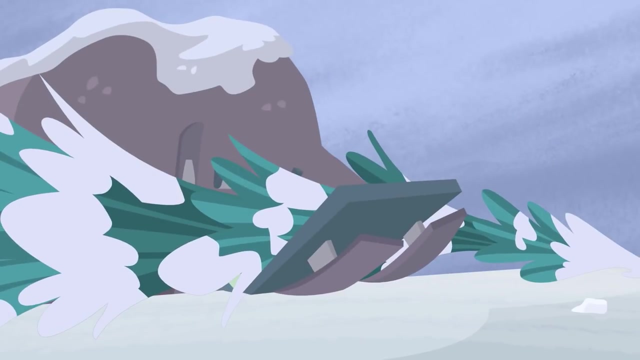 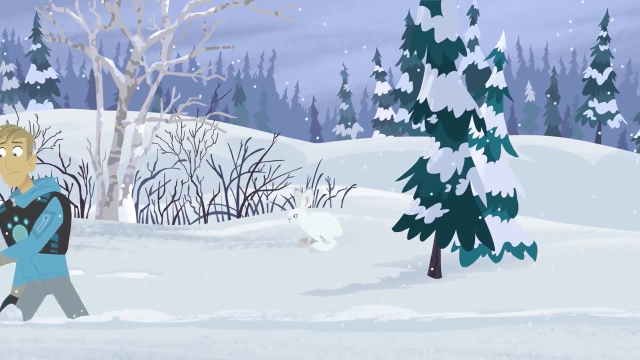 Let's go. There's the gage Break. Uh-oh, Whoo, It's okay, Oh Or not. Well, that sled was good while it lasted. Whoa now. that's a creature built to handle the winter. 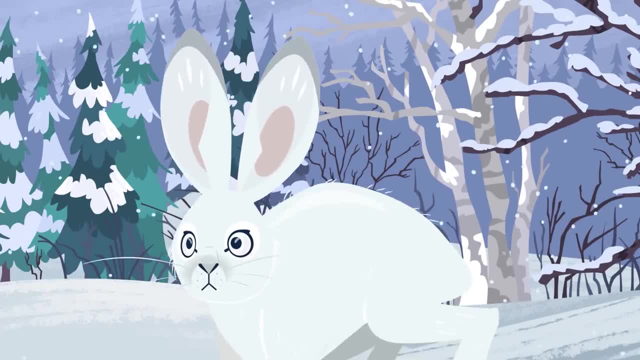 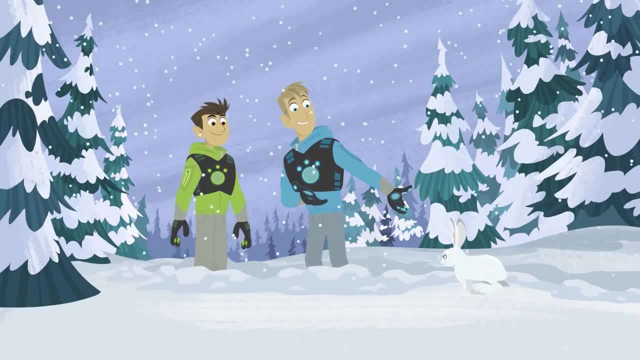 A snowshoe hare. Yeah There, Amazing. He just walks right on top of the snow. He's a snow walker. Look at those huge feet. That's what keeps him from sinking in. Whoa, What's up? Avalanche. 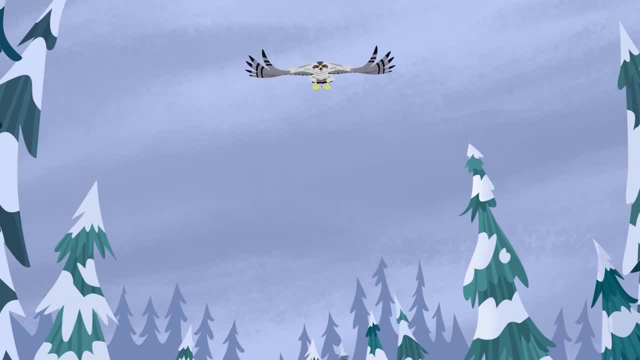 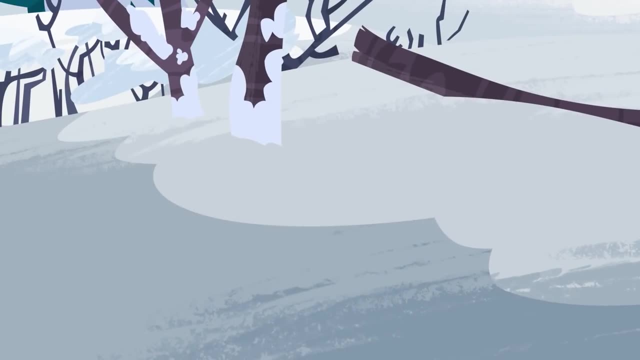 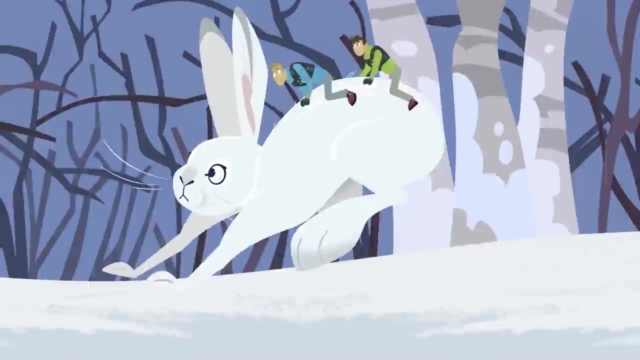 That's what's up. Goshawk Go, Avalanche Go. Those are some powerful legs. Zero to 56 kilometers per hour in just a few seconds, And they still stay on top of the snow without sinking in. It's like a bucking bronco ride. 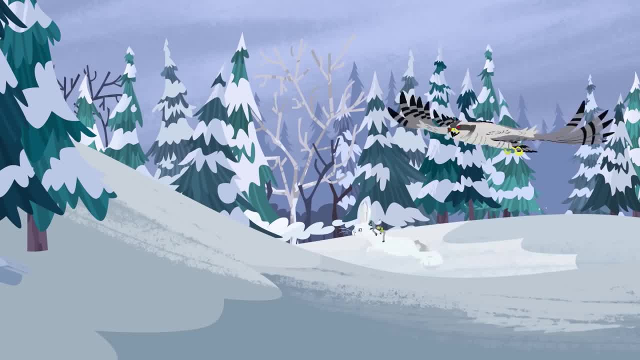 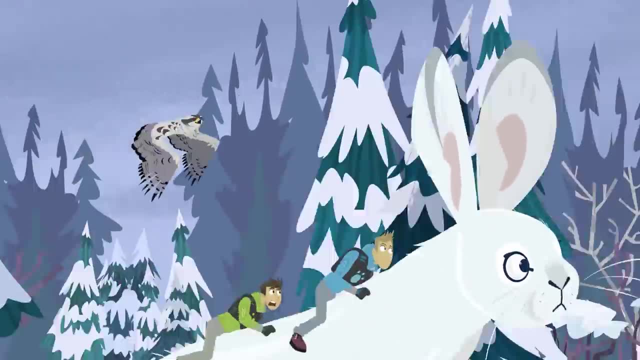 A hip-hopping hare ride. Woo-hoo, Look out. Whoa, Nice seeing you. Avalanche Goshawks, Hawks in general. They're one of the snowshoe hare's worst nightmares. Uh, not exactly a sweet dream for a mini-crat brother either. 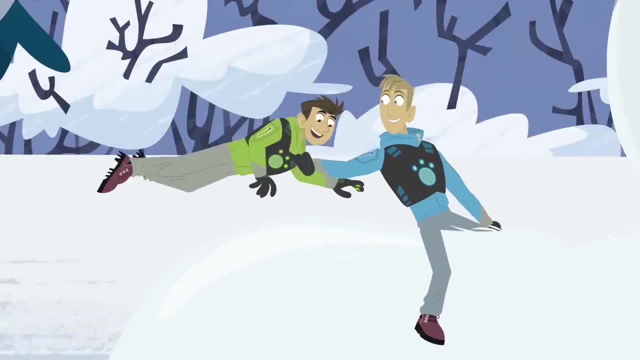 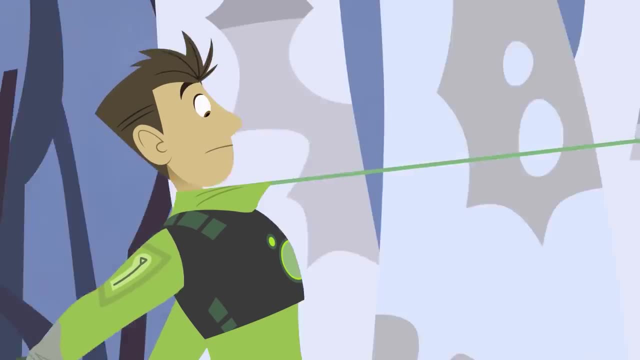 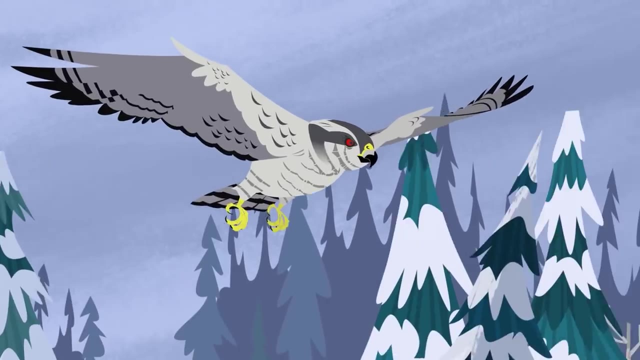 Whoa Ah, Gotcha. Whoa Ah, Whoa, Whoa Ah Ah, Go, go, go, go. He's gaining. He's gaining Whoa. Yes, We're heading to the safety zone. 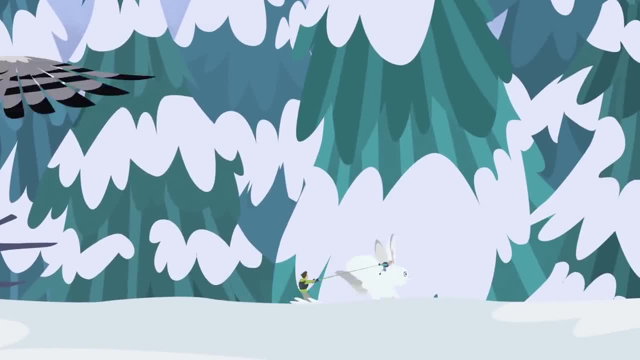 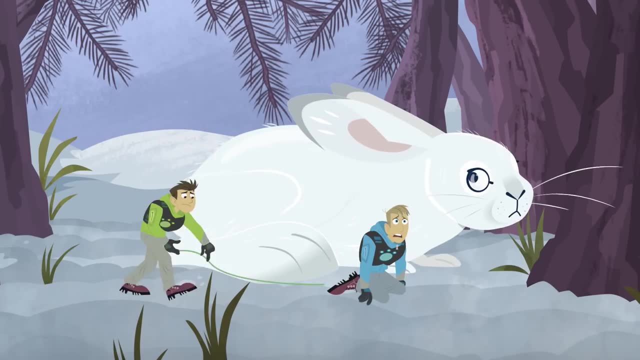 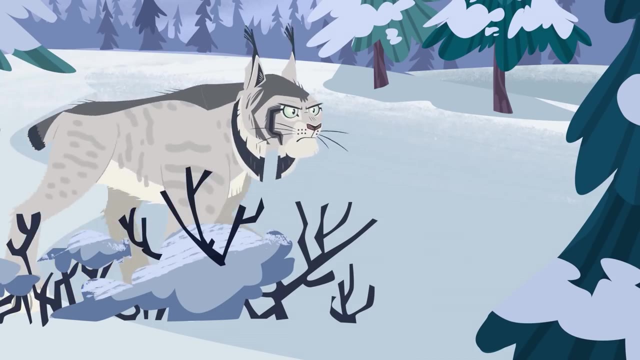 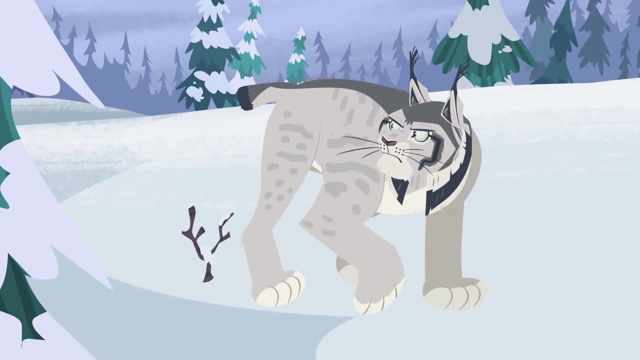 Hang on, Chris. Whoa, Whoa, Ah, Whoa. You know, maybe this wasn't a great idea. After all, you gotta admire this hare-hunting specialist With that dense winter fur and those massive paws that keep her on top of the snow, just like you, Avalanche. 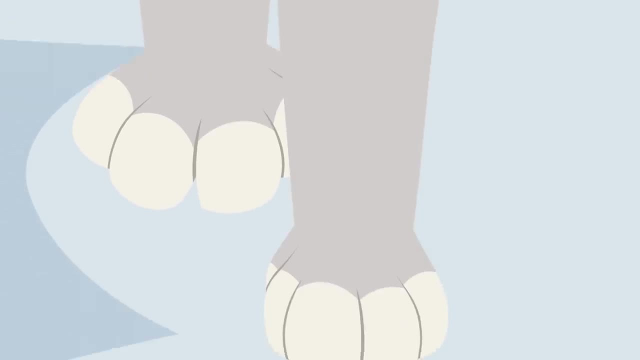 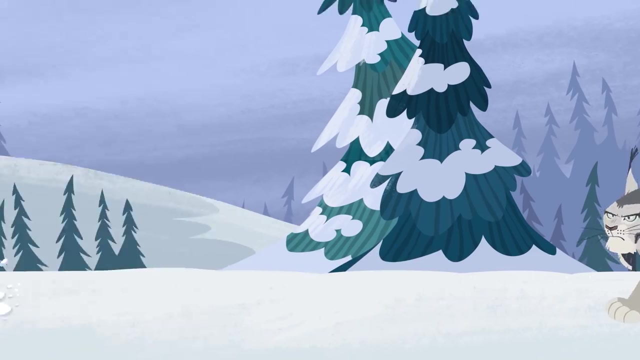 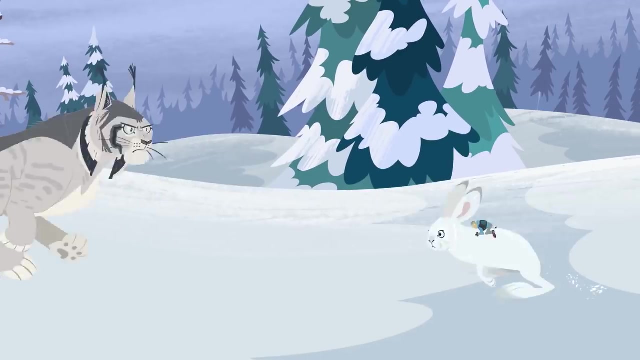 she matches you feature for feature. She even spreads her toes with every step to make them even bigger. Better snow feet. Oh, this is not good. Run, Avalanche, run, Run, Avalanche, run, Look out. Ah, Nice one. 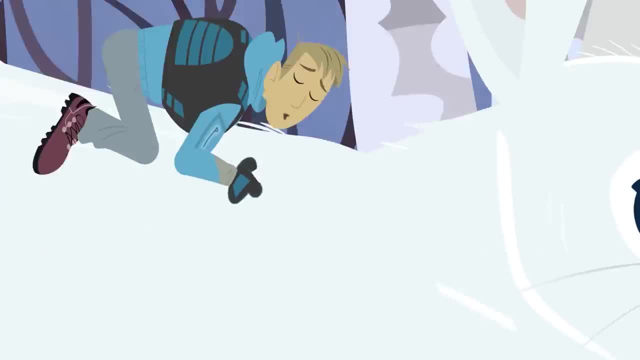 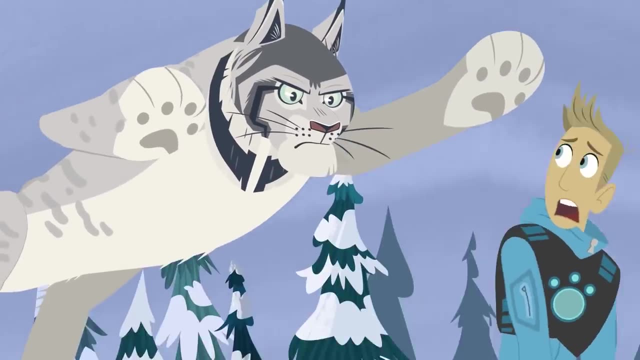 Whoo, The snow-diving technique That bought us an extra stride or two. Yes, the whole thicket Almost there. Go, go, go, go, go, go. Ah, Whoa, Who's had the loose? 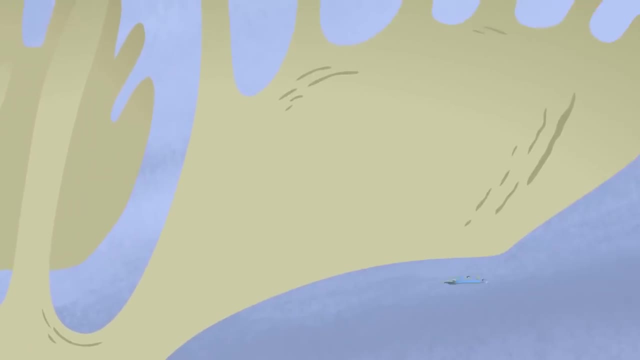 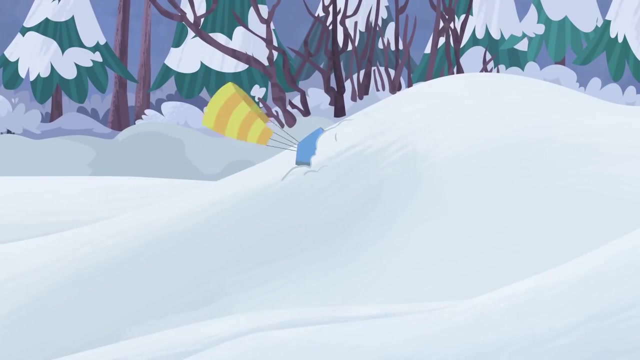 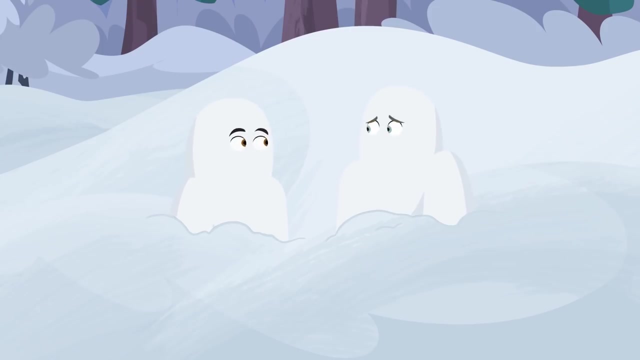 Next place is yours. Next place is yours. Whoo, When we get miniaturized, there are always unexpected obstacles. Oh, Oh, too late. Well, at least we landed in soft snow, Freezing cold, but soft. Yeah, but I think Jimmy just swallowed the flight module. 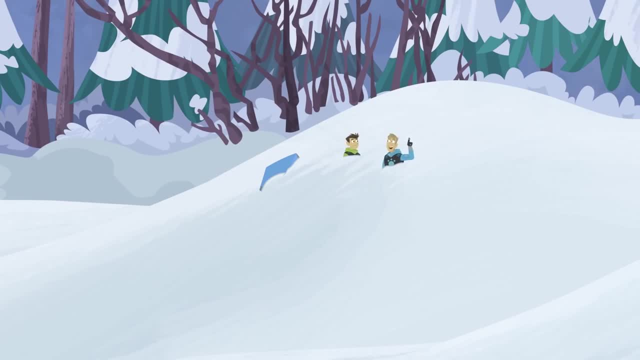 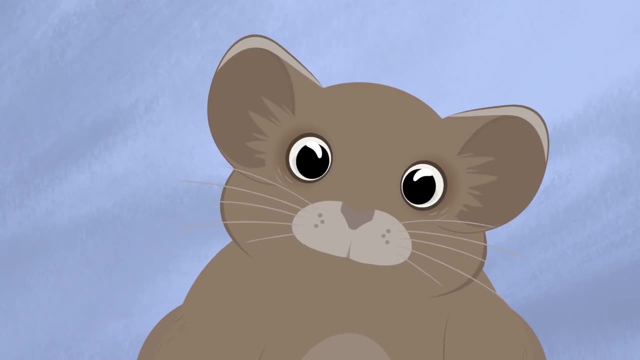 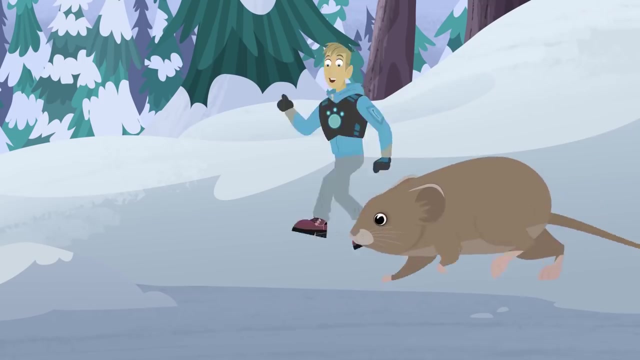 Ah, we're grounded. Good thing Aviva added ground gear. Great, Let's go back to the Tortuga. They'll be waiting for a meadow vole, Kind of like a mouse, but different, shorter tail, A little like a mole, but different, small paws. 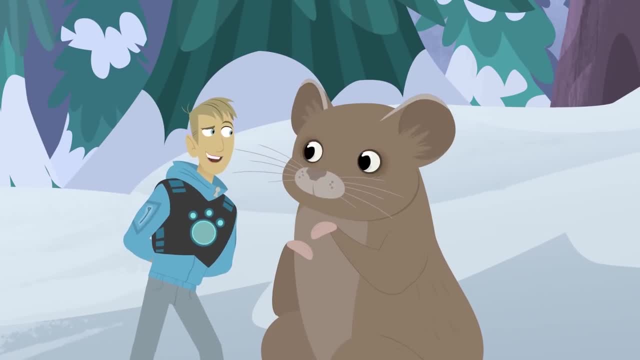 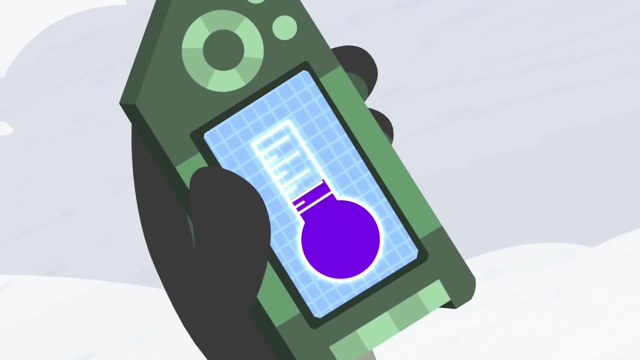 100% vole And pretty roly-poly. Hey, I'll call you Rojo, But what are you doing out and about? It's super cold out, Way below freezing. You should be hibernating or something, Yeah. 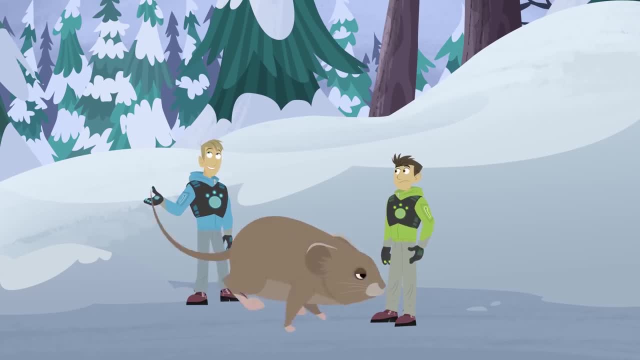 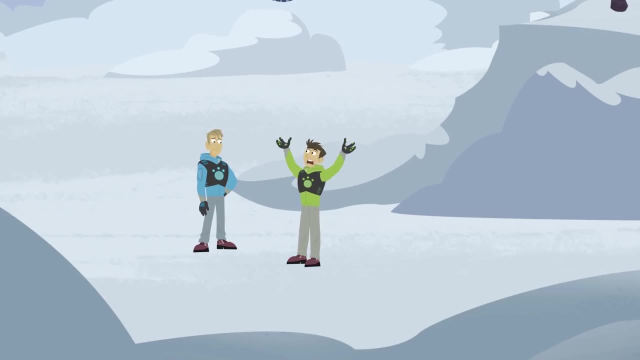 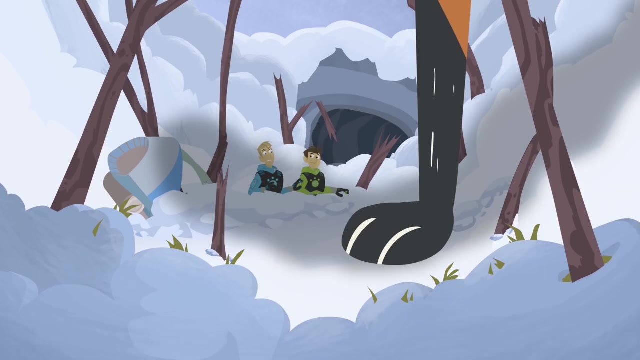 It's winter like groundhogs and bats and hedgehogs, Winter's harsh Freezing temperatures. food scarce, no leaves, no berries. Little guy like you could die out here. Rolo, Wait, hold up. Uh-oh, this paradise just became a nightmare. 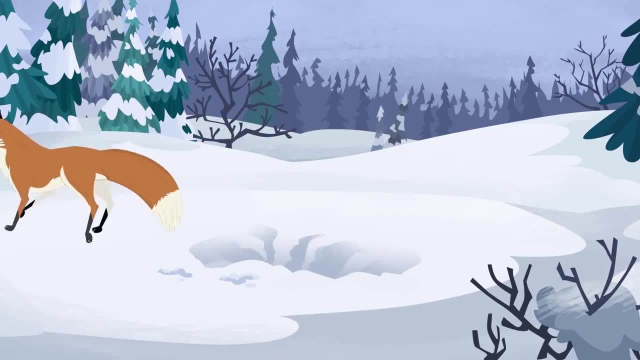 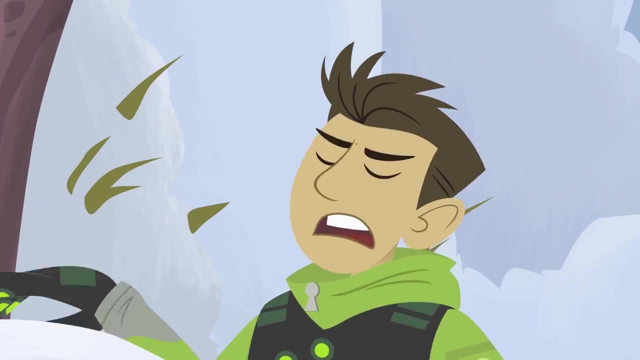 Predators know about this Omnivian Zone too. This is crazy. If we're having a peaceful time down here, then boom, It's all over. I know Anything Could be listening from up there, Listening for the voles skittling around and chewing. 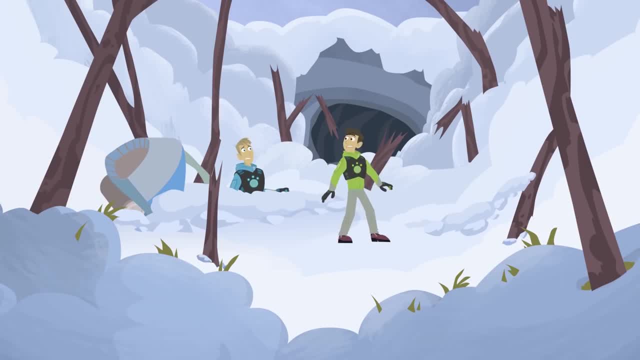 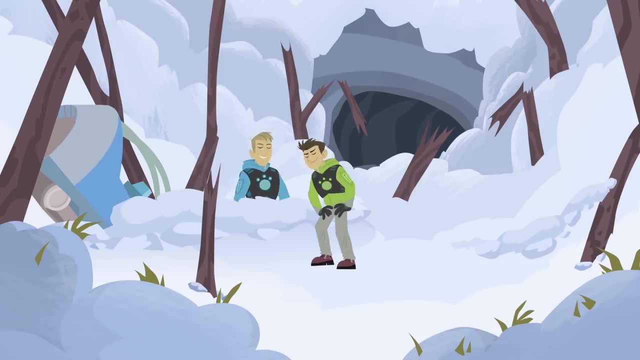 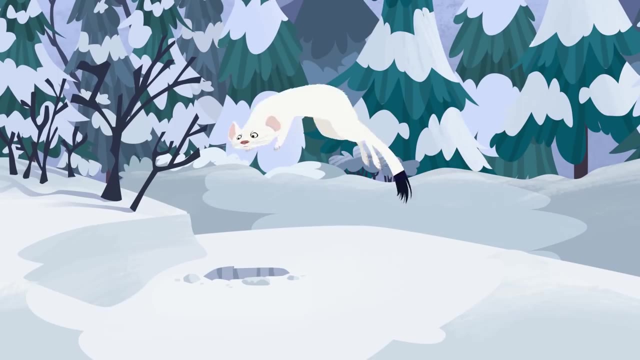 As long as no one makes any sudden loud noises, we should be fine. Ah Shh Ah, Ah Shh Ah Ah. Chew Chew, Chew, Chew, Chew, Chew. Oops. Hopefully nobody heard that. 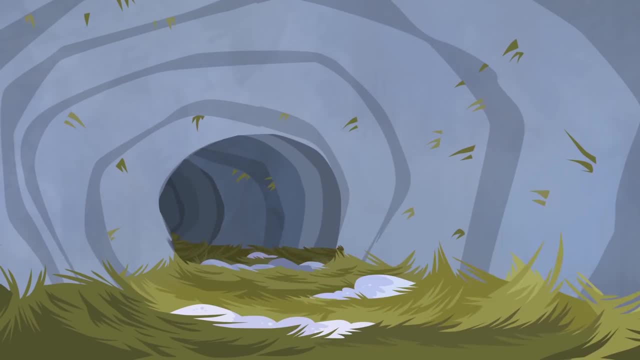 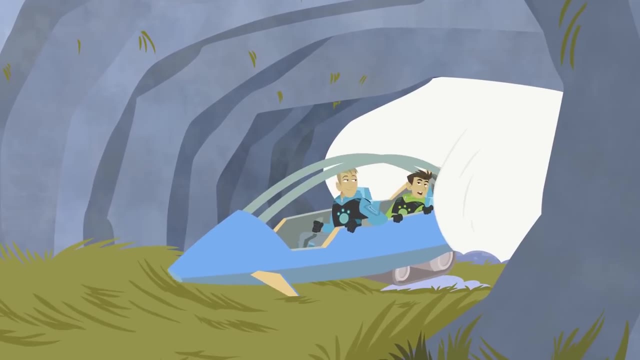 But let's get out of here anyway Quietly, Martin, Drive quietly, We'll see you, Rolo, It's been fun Quick. let's get out of here, bro. Oof, Huh, Where'd that snowbank come from?